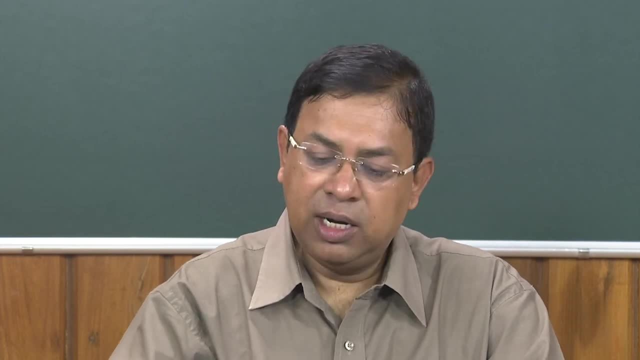 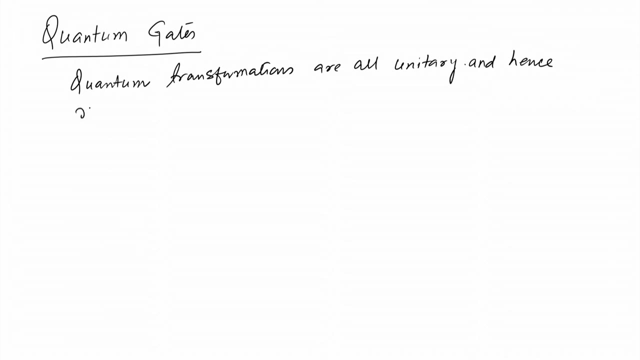 an angle pi. So so these are reversible. So let us, and very importantly, 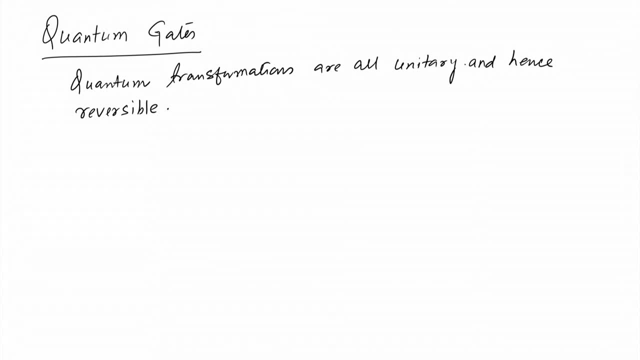 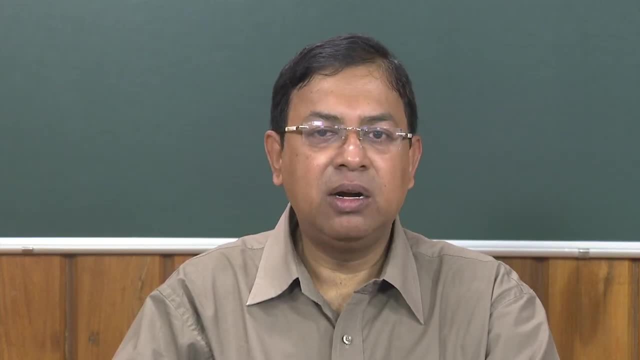 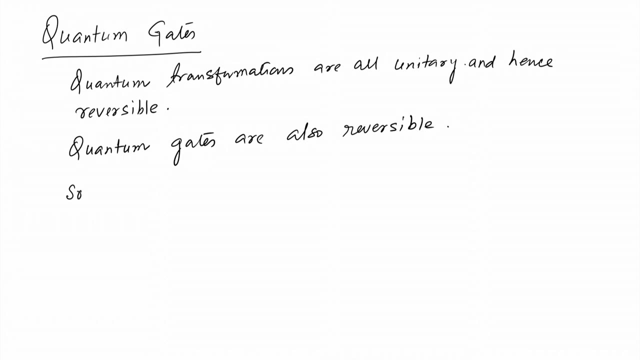 So we will discuss some of the simple quantum gates that are used, or rather useful, for the single qubit quantum state transformation. So we will look at this for the single qubit and then we will also discuss 2 qubits and briefly on multi qubits as well. So this is I, is an identity transformation will tell. 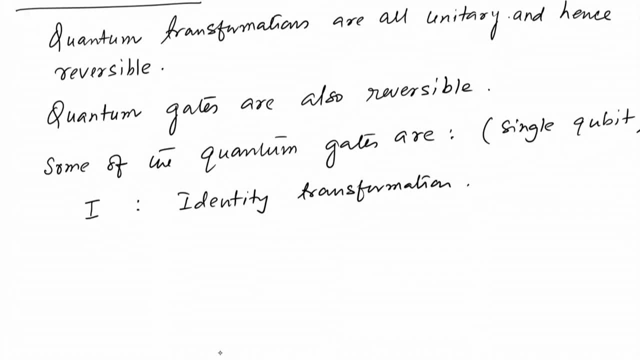 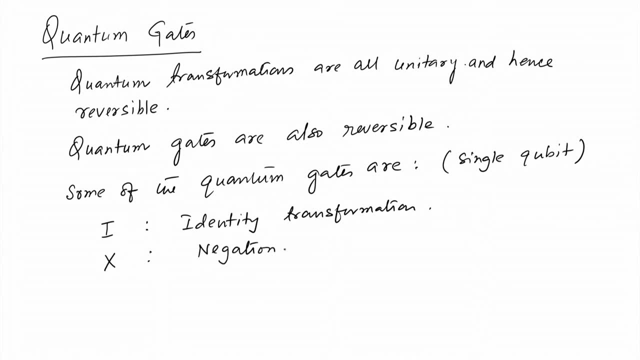 you what it means. and then x is called as negation, and then it is z which is called as phase shift- We will just give the forms of that- and y, gate, which is a combination of z, x. that is a combination of phase shift and negation. So what do we mean? 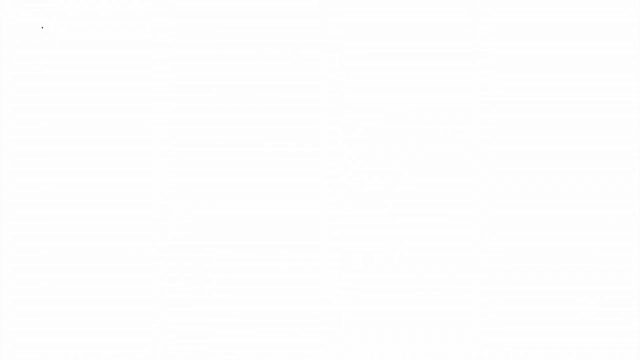 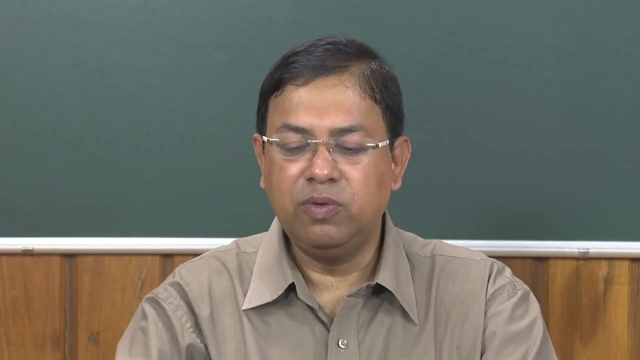 by that. Let us see so the identity i that on a 0 gives a 0, on a 1, it gives a 1. ok, So this has a form which is 1001,. so if it, this is in the standard basis of 1 and 0, in which 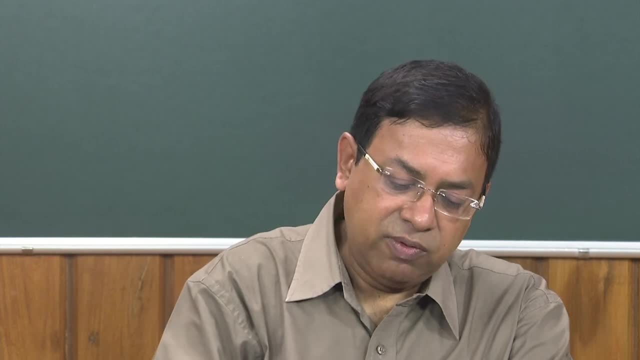 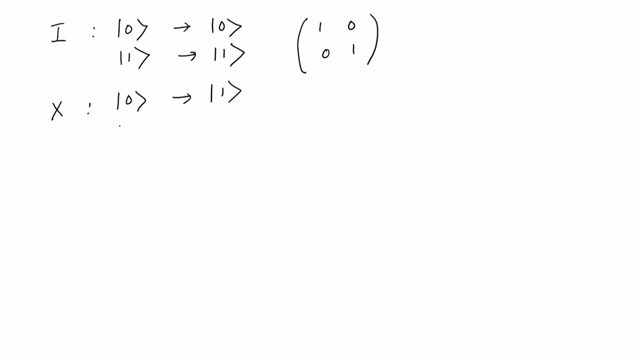 the qubits are represented, And then we have x: 0.. Steriot: 0.. S 0.. GA x: x 0.. S 0.. x. acts on a 0 gives it a 1 and acts on a 1 gives it a 0. So this is a negation and this is. 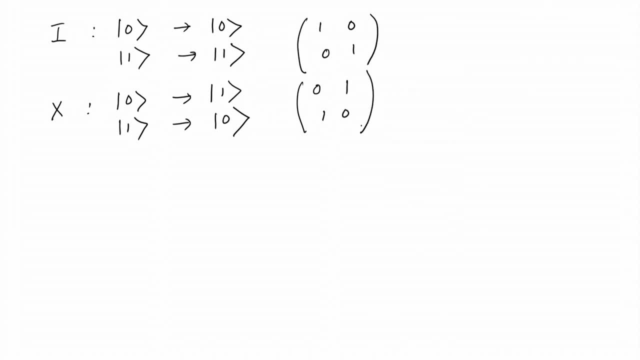 0, 1, 1, 0.. Then let us write z, which acts on a 0, gives a 0, acts on a 1 gives a minus 1.. So this is written as 1 0, 0 minus 1.. Remember that x gate looks like Pauli matrix for kind. 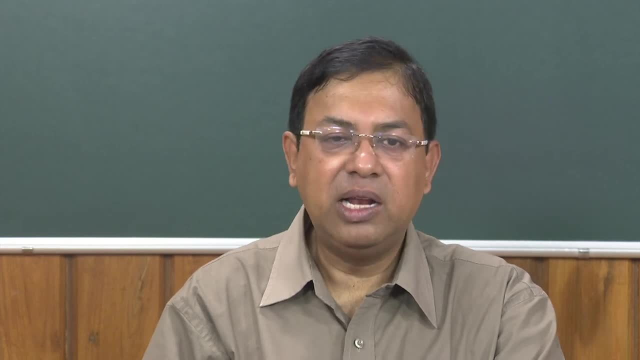 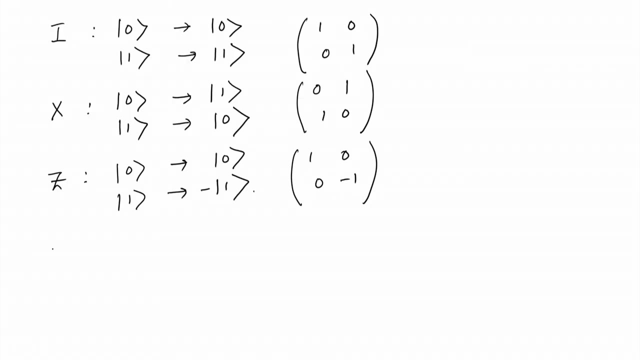 corresponding to the x component for a spin half particle and similarly z looks like a sigma z for a spin half particle again. And now the combination, which is y is: it acts on a 0, it gives a minus 1, and it acts on a 1 and it gives a 0. So this is nothing. 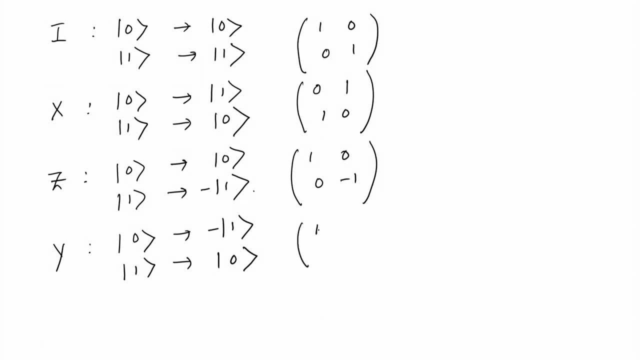 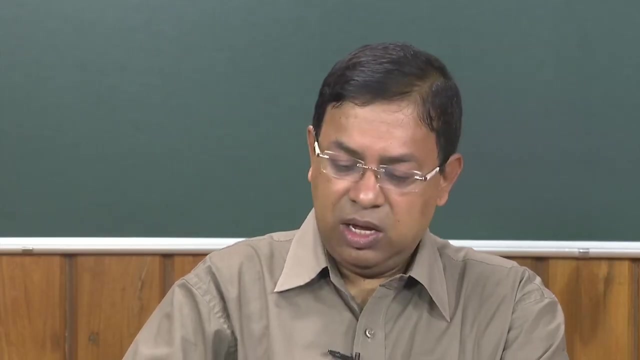 but equal to 0.. 1, 0 0, 1 minus 1, 0.. So this is almost like the sigma y, the y component of the Pauli matrix, excepting for a lack of a imaginary i. So all these things are unitary, which. 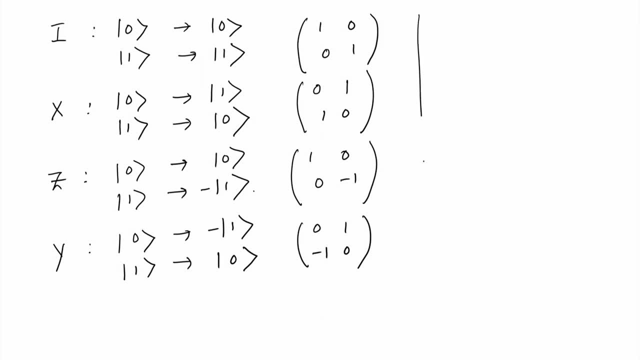 can be checked individually, For example. So either you do a x transpose x, that will give you a unitary matrix. Similarly, a Y Y transpose also gives an unitary matrix, and so is true for others. So these are some of the things that are the single qubit gates that are important. 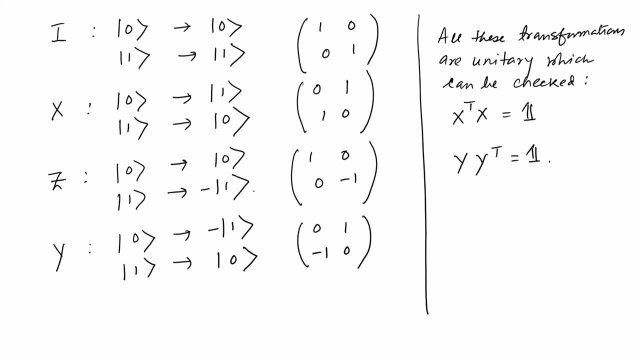 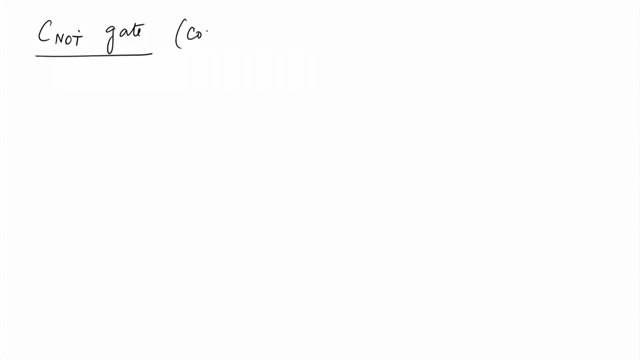 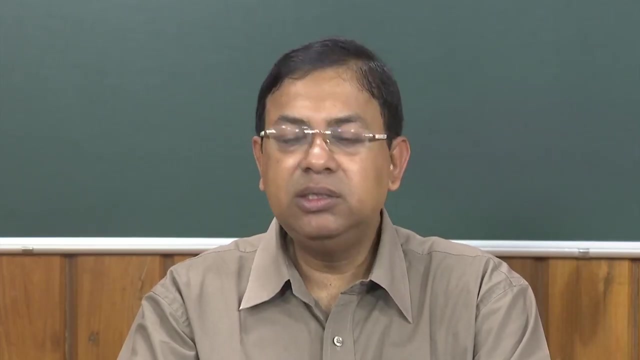 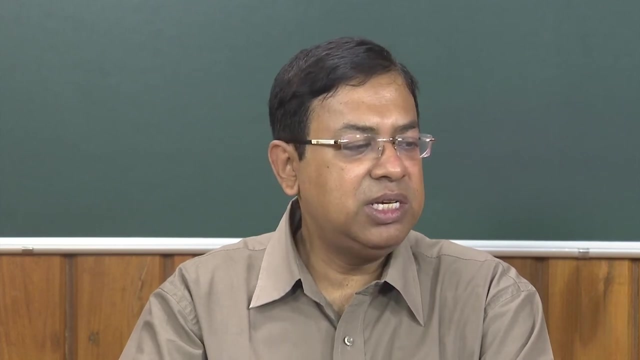 C naught gate. C naught gate And the full name is called a controlled, not gate. This was used while we discuss the quantum entanglement, and then a simple variant of that we have used in quantum teleportation, which we called it as C x gate. This is called as a C naught gate And if this operates on, 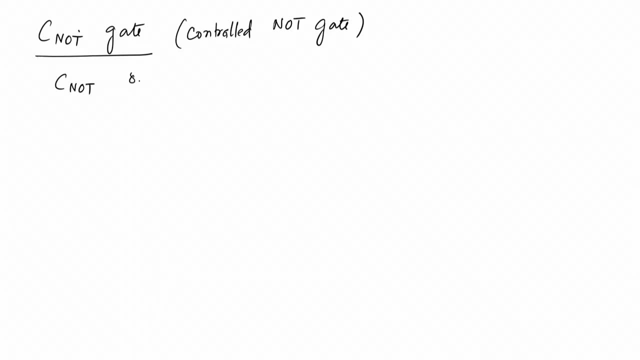 C x gate. C x gate- Basically a 2 qubit system and the rules are so. it changes the second qubit if the first qubit is 1, else does nothing. So what it means is that. So, as I said, 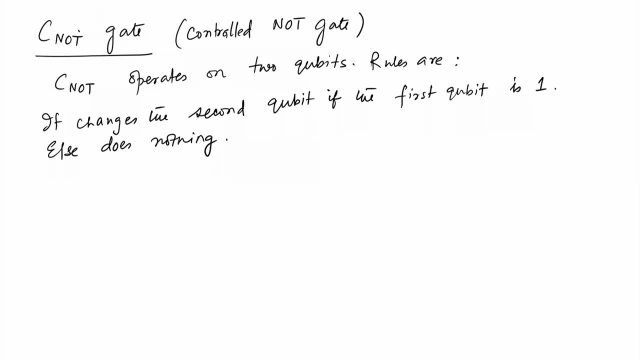 So, as I said that this is like this CX operation or the C naught operation that we have seen earlier, So for a 2 bit, the space is So this is like 0, 0, 0, 1, 1, 0 and a 1, 1.. 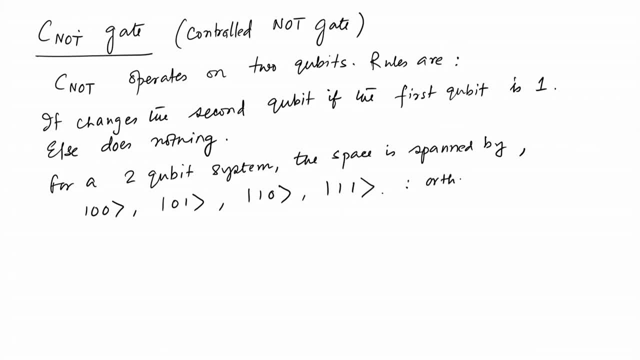 So this forms the basis of that. So this, So this, So the C naught, So the C naught On a 0, 0.. It Transpts 0, 0 on a 0, 1, it is just keeps it unchanged. that is 0, 1, 1, 0, since the first qubit is 1. 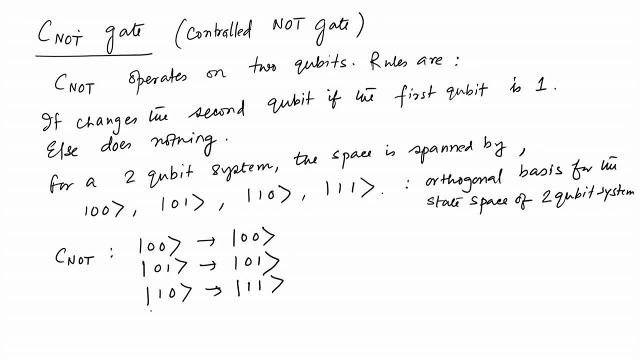 it will change the second qubit to 1 as well and similarly 1: 1, it does it 1: 0, because the first qubit is 1, then the second qubit is changed to 0.. So the 4 by 4 matrix form is: 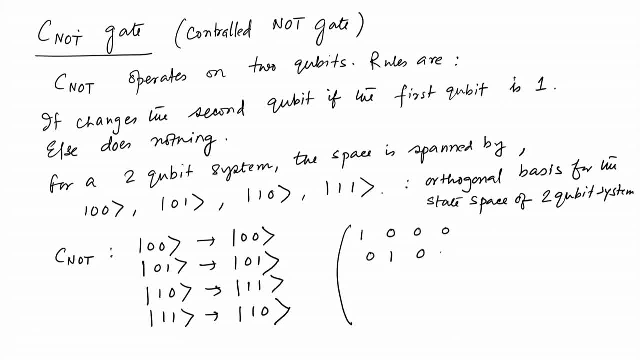 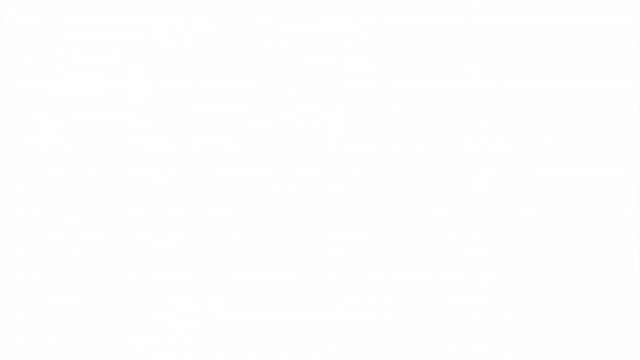 1 0 0 0, 1 0 0 0 0 0. 1 0 0 1 0. So that is the matrix form of this CNOT gate and one can change it. So we can check that CNOT is a unitary transformation by checking that CNOT transpose or CNOT which. 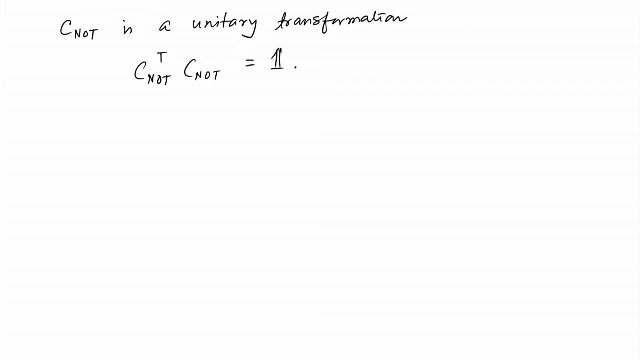 is equal to an identity matrix. So, in principle, the CNOT is, or rather it is, It cannot be. is not a tensor product of 2 single bead transformations? ok, So it cannot be represented as a tensor product of 2 single cubit transformation. Let us look at the graphical 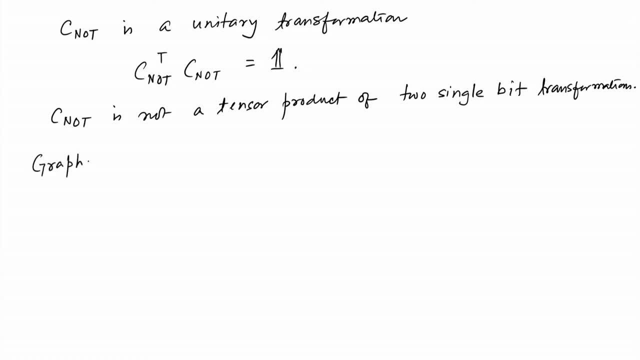 representation of this gates. So usually it is a box, the single cubit ones. they are by 2 lines, So this could be x, or it could be, you know, z, for example, or y. So it is just a box with 2, one line going in, the other line going out. However, there is a, the c, 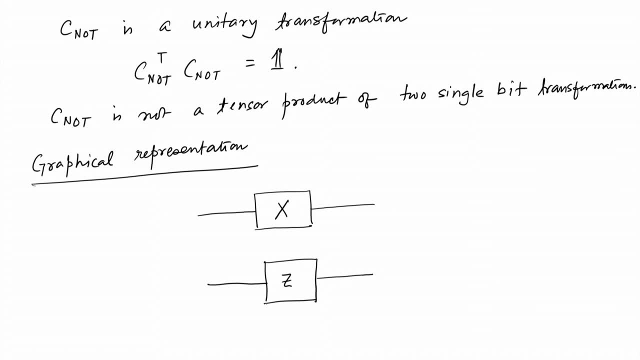 naught gate has a slightly different form than this, So it is a 2 lines and open circle here, a vertical line with a crossed mark. So this is the, so the open circle, So this is the open circle and this is that cross mark. The open circle indicates that there 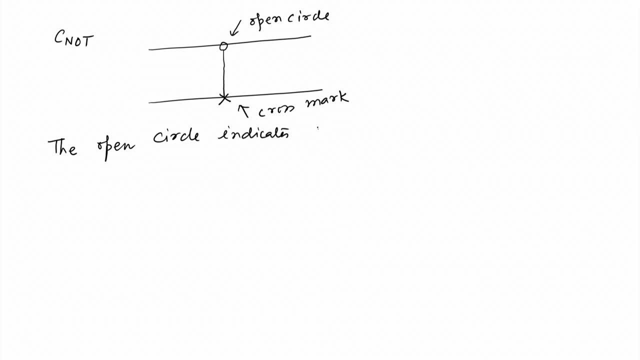 is a control bit and the cross mark indicates the control bit and the cross mark indicates the conditional negation. So the single cubit transformations are replaced or represented by just a block, a box and 2 lines on either side, and c naught gate is represented by 2 horizontal lines. 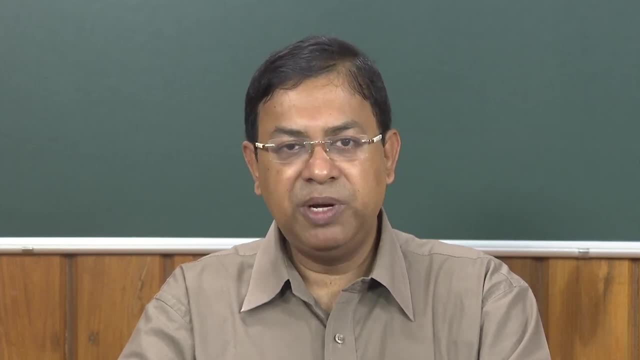 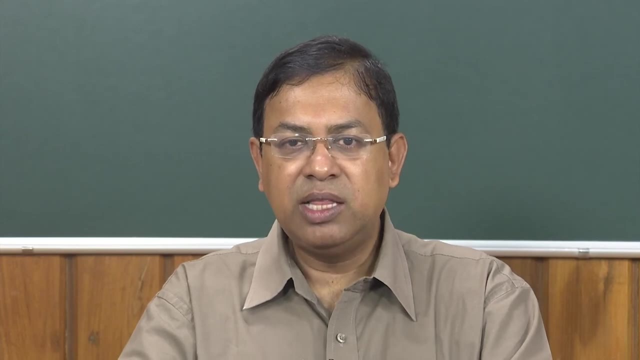 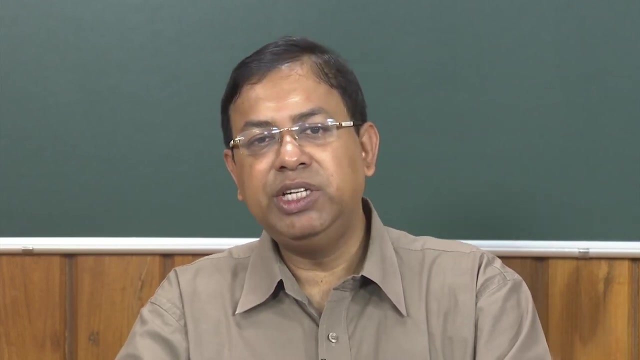 with an open circle control bit and the x mark which is at the bottom of a vertical arrow starting from the open circle. that represents there is a conditional negation, that is, if the first bit is 1, then you change the second bit and if the first bit is 0 then you do nothing. 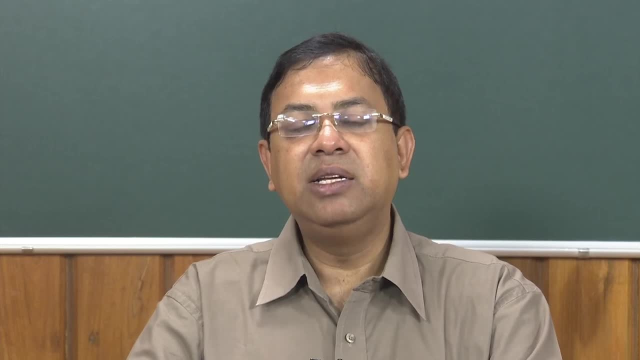 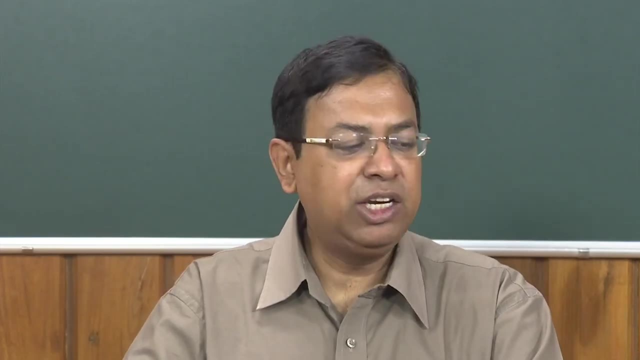 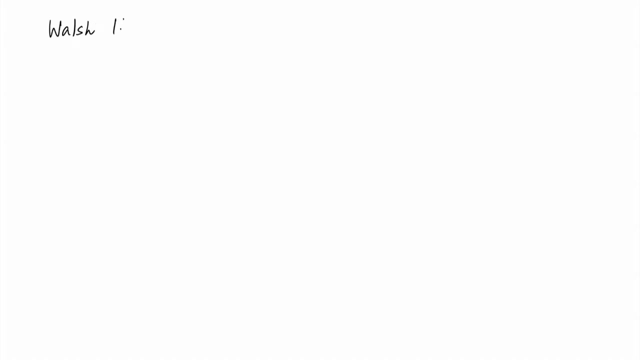 So we have looked at so far the single qubit and the 2 qubit transformations. Let us look at a little more complicated, that is, at n qubit transformation and this called as the Walsh-Adamard transformation. So we have looked at the earlier the. 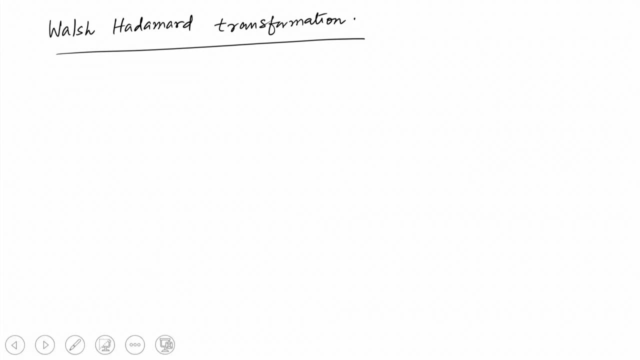 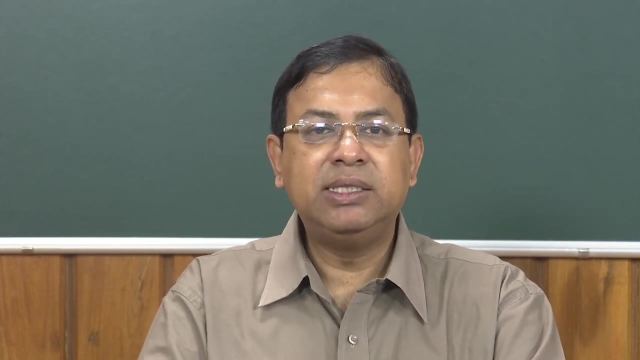 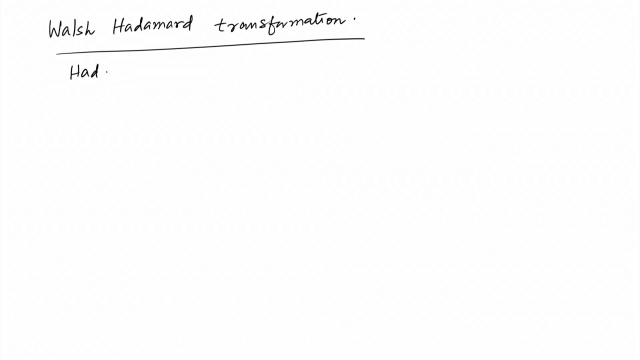 5 transformation. So this is an important transformation on the single bit, because a single qubit is now represented as a combination of, or superposition of, 2 bits. So ok, So on a single bit and transforms into a superposition. 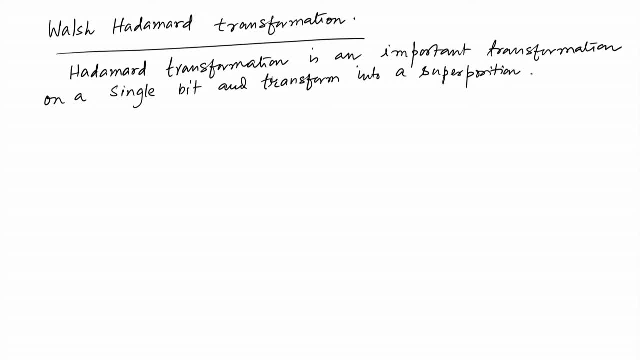 Ok, So H is represented by H which, on acting on a 0,, it is a normalized superposition of a 0 and 1 and on a 1, it is just a change in sign for the second term, which is also superposition like this. 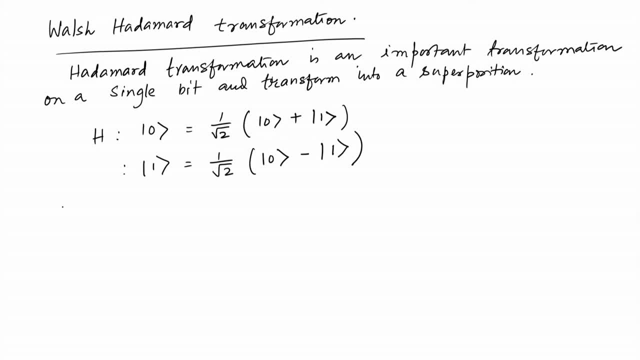 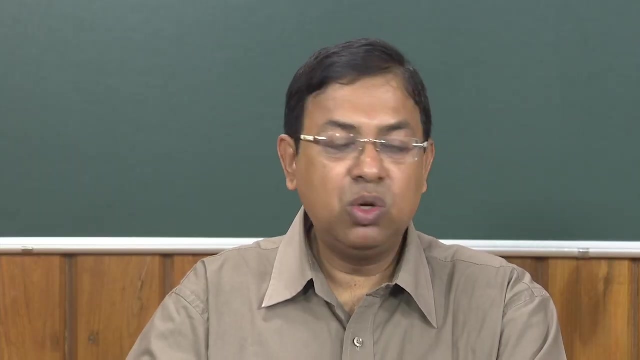 So this has, So this has important applications applied to 0 and 1.. So all these Earth 1 can create a superposition, alright, So this can in principle be applied to n bits, So H can actually generate a superposition of all true to the power n possible states. 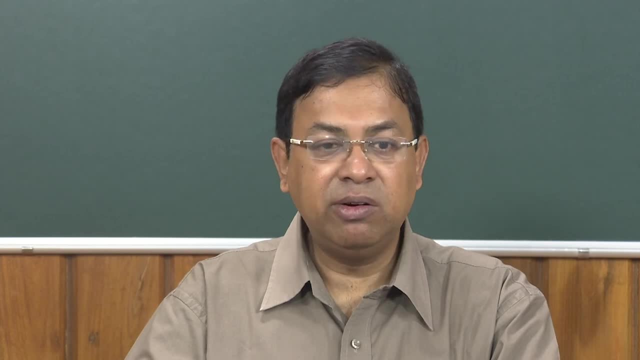 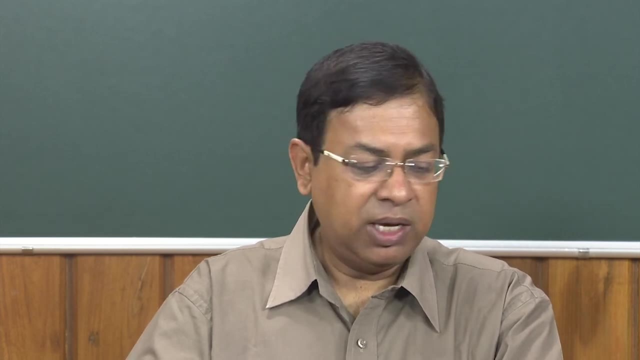 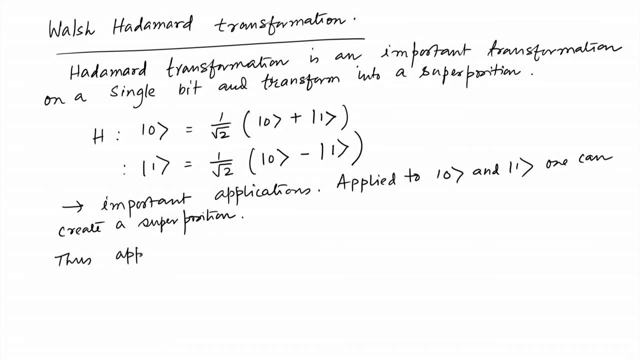 n possible states, which can be viewed as a binary representation of the numbers between 0 to 2 to the power n minus 1.. Let us see what we mean by that. In fact, this is an important statement, So let me write it down. 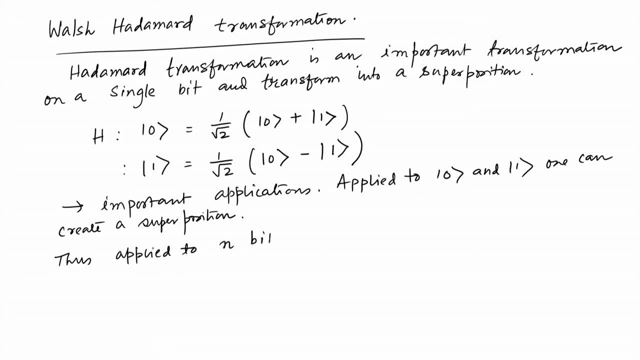 Thus, applied to n bits, H can generate superposition of all 2 to the power n possible states which can be viewed as binary representation of numbers from 0 to 2 to the power n minus 1.. So what this really means is the following: 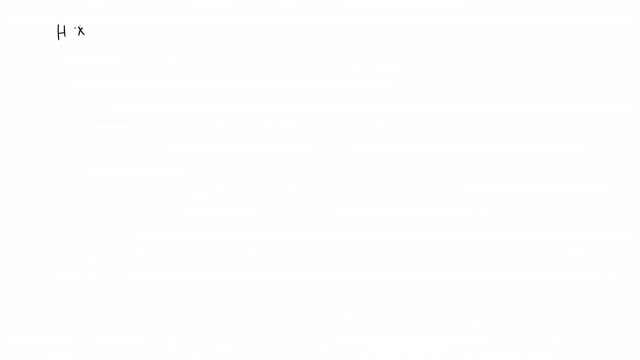 that this Hadamard transformation being applied successively to this bit n bit system, this will create a 1 by 2 to the power n and each one will create, as we know, that it is 0 plus 1, then a tensor product of 0 plus 1, and so on, and then it. 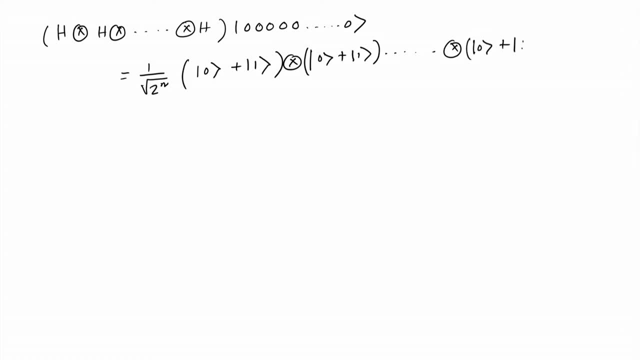 is n by 2 to the power n over x, 0 plus 1. ok, So this is the successively applying this, and this is called as sum over x equal to 0 to 2 to the power n minus 1, and we will: 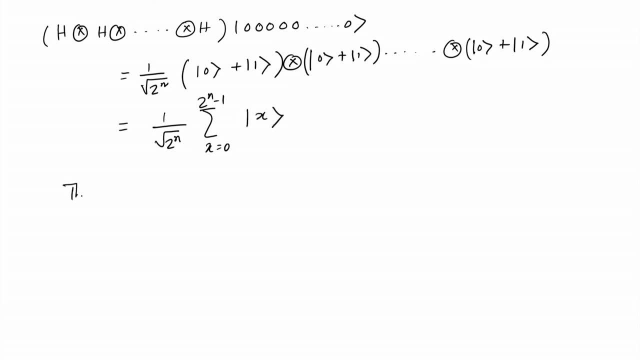 write it as x, So this is called as x: 0.. 2. 1. 0.. 2. 0.. Walsh-Thomard transformation and it is represented by a W. where it is a, it is a W is a recursive. 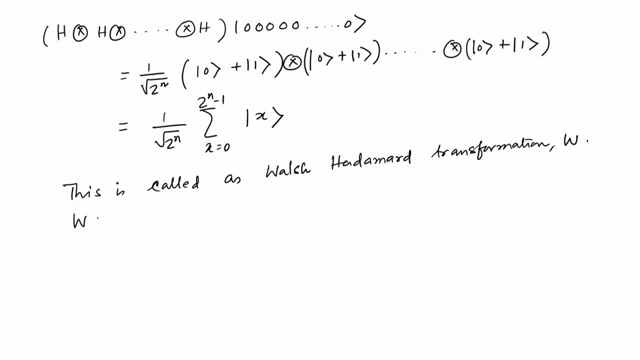 W is a recursive decomposition of the form. So W 1 equal to H and W n plus 1, that is H and the tensor product of W. So this is how multiple quantum bit, or rather multiple bits, are being superposed, or rather: 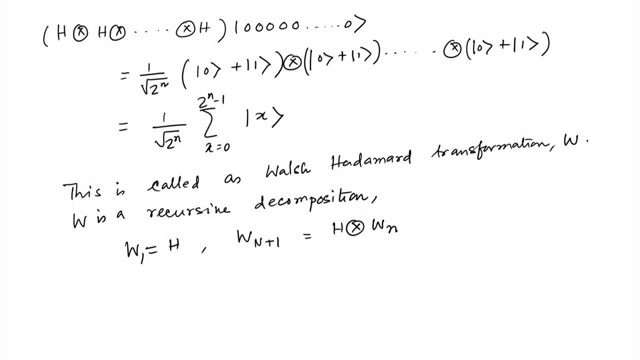 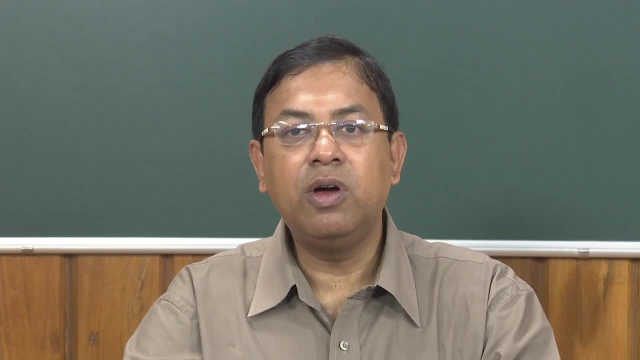 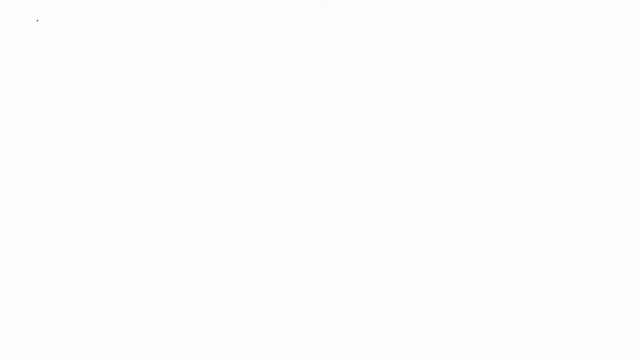 they are. you know this Walsh-Thomard transformation that creates a state which is a tensor product of multiple bits. Let us now look at another important thing, which is called as a no cloning. So the unitary property of the quantum states say that they cannot be copied, or rather cloned. So let 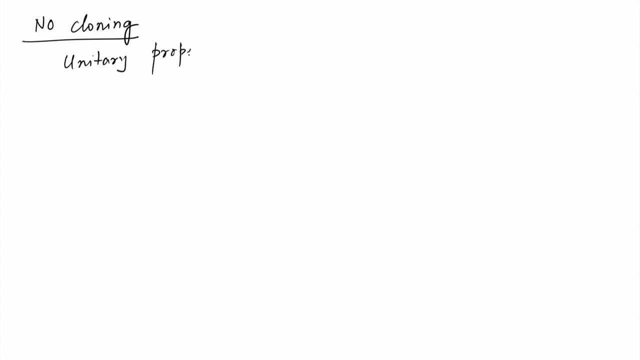 us code, a storing heap of points, and then call it a no cloning. Now, basically, the quantum states cannot be copied, or in this language, they are also called as cloned. So we give a very simple proof of no cloning. no cloning theorem. ok, Suppose u is a unitary transformation. So 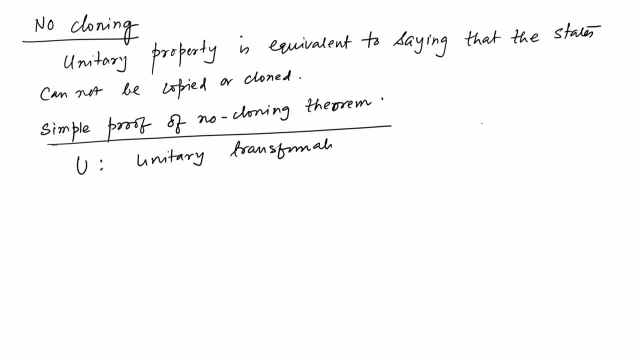 a unitary transformation which acts on a state A- 0 and creates a state A- A for all quantum states A. And let us have another state, orthogonal state B, quantum state B, where it is an orthogonal to A. So this is equal to 0, and so the so? u on A 0 creates A A and u B 0 also creates. 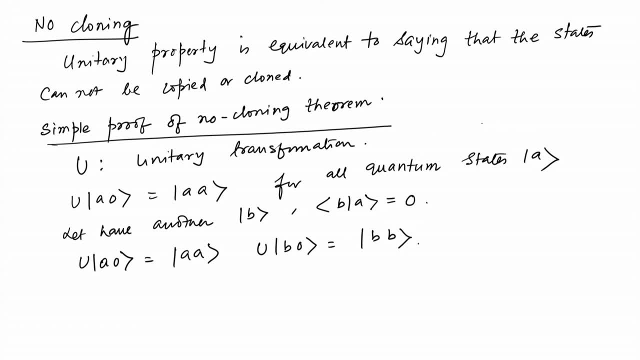 a, B, B. So let us say: let us have a, C, B, C, which is equal to 1 by root, 2, A and B, the superposition of A plus B. So that is a new state. this is by linearity. 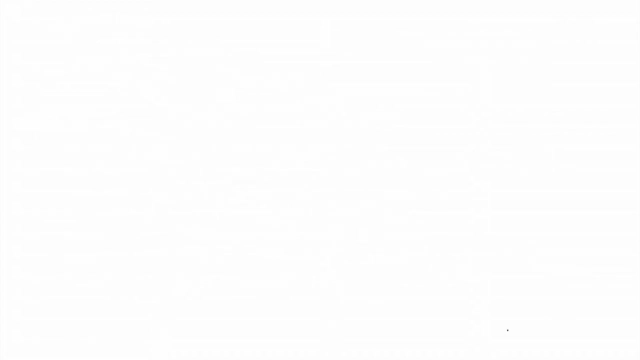 Now what happens is that u? u on u on C 0, so this would create 1 by root 2 and then u acting on A 0 plus u acting on B 0. that is going to give a 1 by root 2, A, A plus a, B, B. ok, 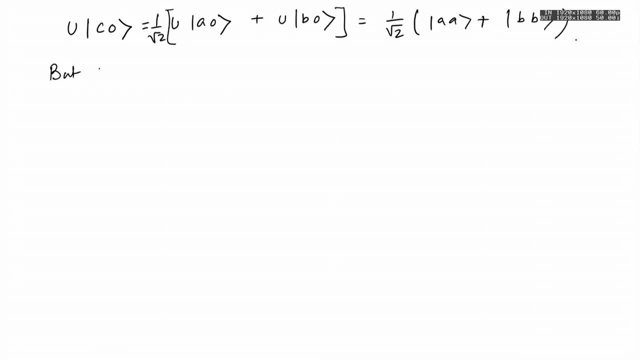 But if u is a cloning transformation, then u, acting on C 0, should be giving me a C, C which is equal to 1 half of A A plus C 0.. Ok, So this is a cloning transformation. Ok, So this is a cloning transformation. 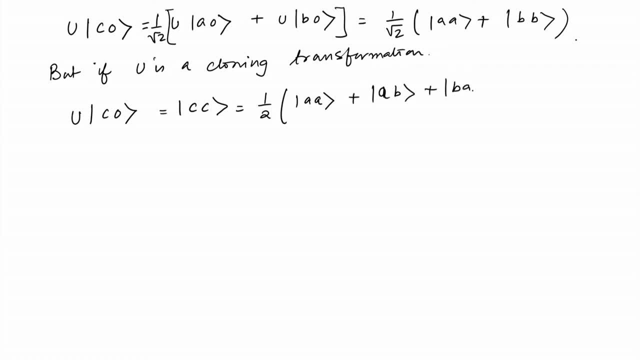 So this is a cloning transformation, So this is B plus a AB plus a BA plus a BB, which is certainly not what we have written above. So these 2 transformations do not agree. So, basically, what So? So, basically, what it says is that there are no unitary transformations which that can. 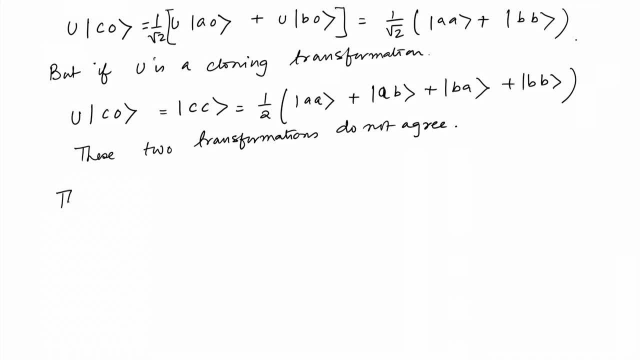 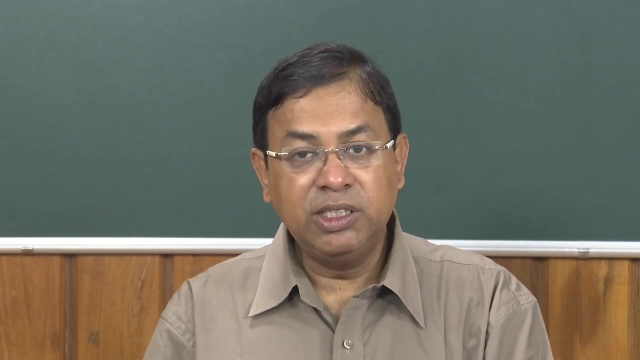 clone an unknown quantum state. So let us box this, because this is the statement of the proof that we had just given. So it is clear that the cloning cannot be done by measurement, because measurements actually are probabilistic And not only that, they are destructive as well. So they destroy the states which are not in the subspace of the measuring device. That is, if you want to have a up spin in a certain measurement, it cuts down the down spin for that particular particle. So it is not possible to create. 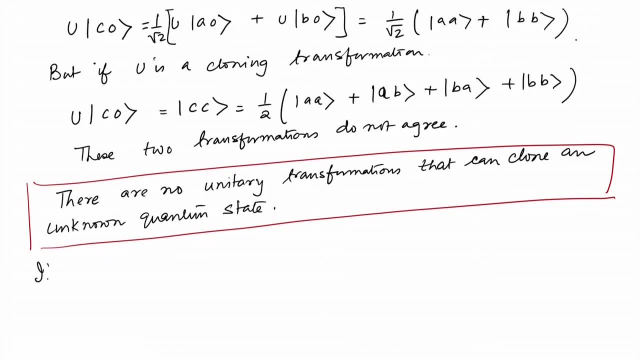 So it is not possible to create …create a end particle state such as a 0 plus a B 1, and a 0 plus a B one, and so on: a 0 plus a b 1, starting from an unknown state. So this is about the quantum computation. 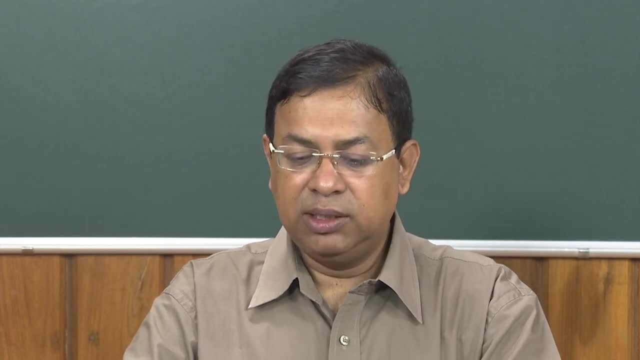 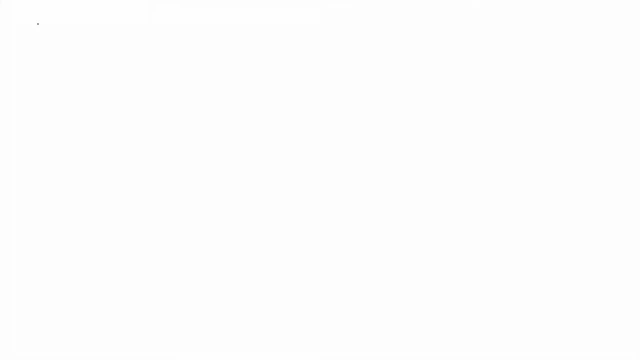 or the quantum information that we wanted to say. just let us have a quick summary of things that have been done, The highlights, rather the highlights of this thing, because we cannot spend a whole lot of time on this quantum computation, because there are other things which are equally important, which are application oriented, or rather they are direct. 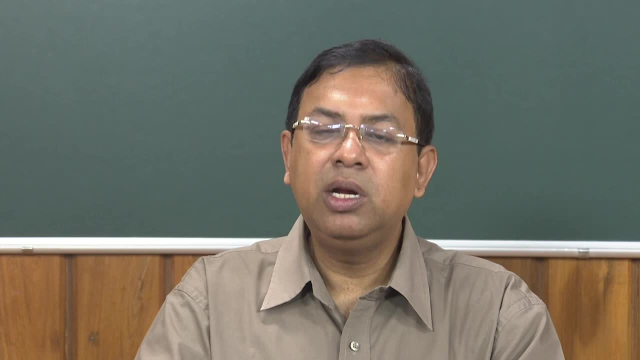 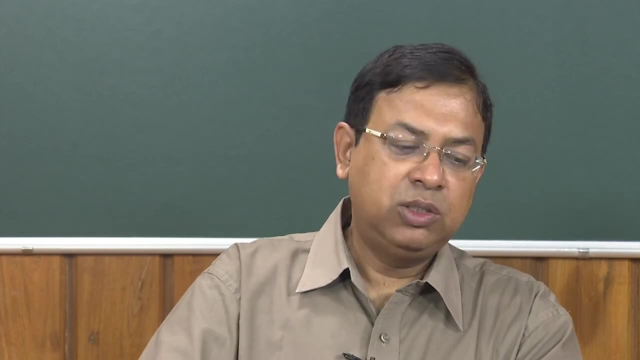 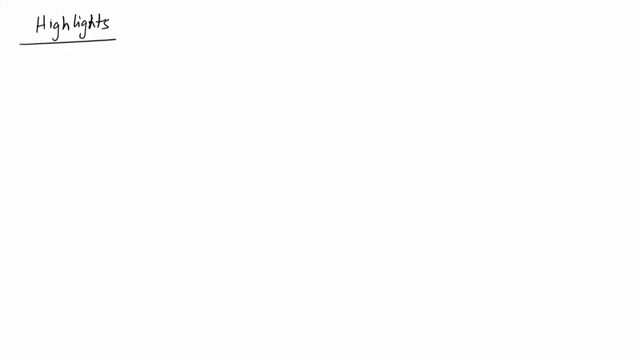 applications of the quantum mechanics that you learn. So we will move on to another topic, such as perturbation theory, but before that let us give the highlights, So the two things that we have done with a lot of emphasis or illustration. one is called as the quantum entanglement. 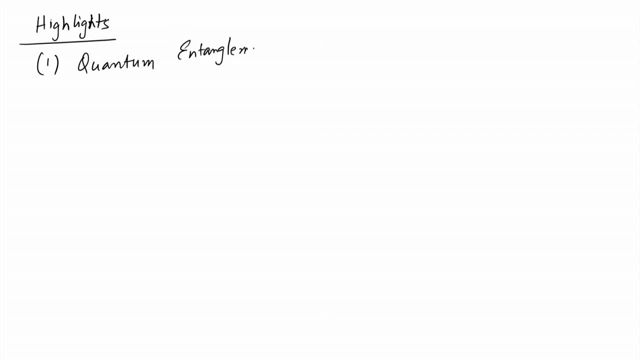 Then it just simply says that the state 0, 0 plus a 1- 1. you can normalize it with a 1 by root 2. it cannot be formed. 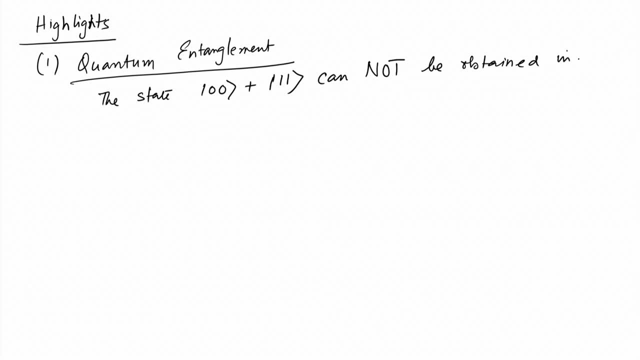 in terms of each of the qubits separately. So what we mean? to say that for no choice, or no choices for A 1, A 2, B 1, B 2, for which one can get get A 1, 0 plus a B 1, 1, and then 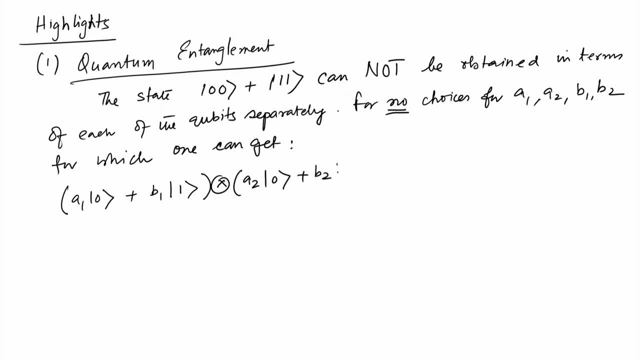 A 2 0 plus a B 2 1,. this will give us 1 0 0 plus a 1, 1.. And the reason is very simple, because this: if you multiply, it will become A 1- A 2 0 0 plus A 1- B 2 0, 1 plus A 2- B 1. 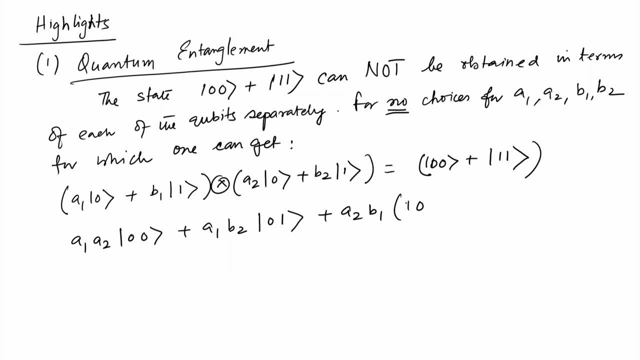 1- 0 plus a B 1, B 2, 1, 1.. Now for these two become 0 then, so for the coefficients need to be 0. So A 1- B 2 has to become equal to 0, or A 2- B 1 has to become equal to 0, in which? 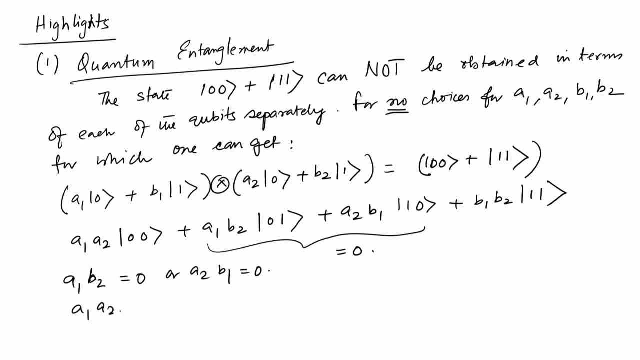 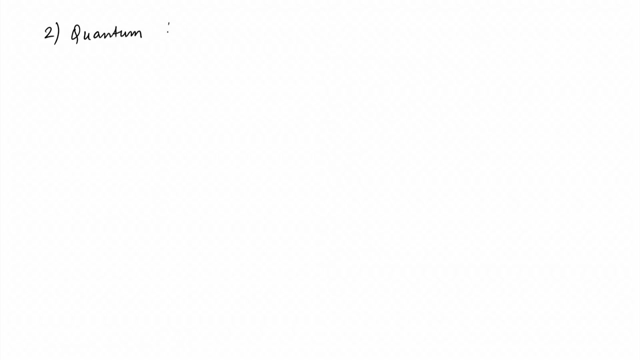 case, either A 1- A 2 will become 0 or B 1- B 2 will become 0, and hence we cannot have a state which is a 0- 0 and a 1- 1, and this called as a entangled state, And similarly for the quantum teleportation. 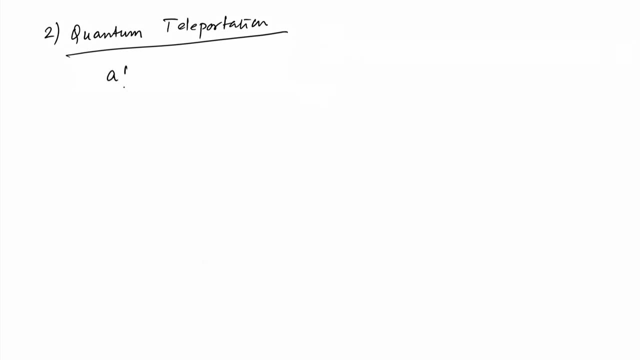 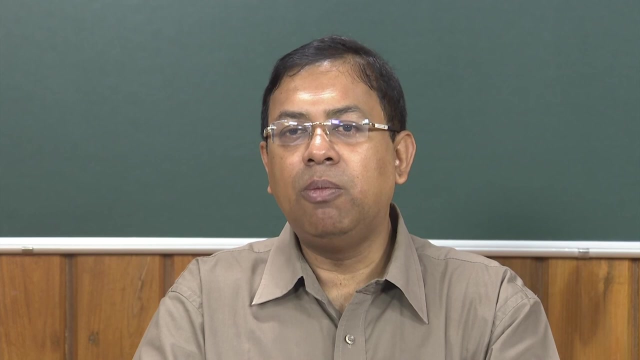 we had spin, So we have a single spin, A up plus a B down that were teleported from lab A to a lab B, which could be separated by universes, which means that this there is no direct linkage from A to B, So that this can be really taken and put it there, but it was teleported. 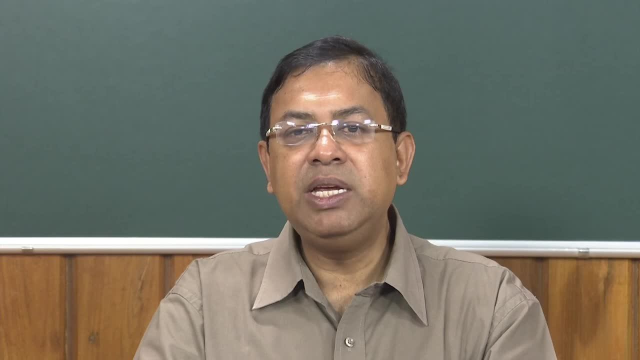 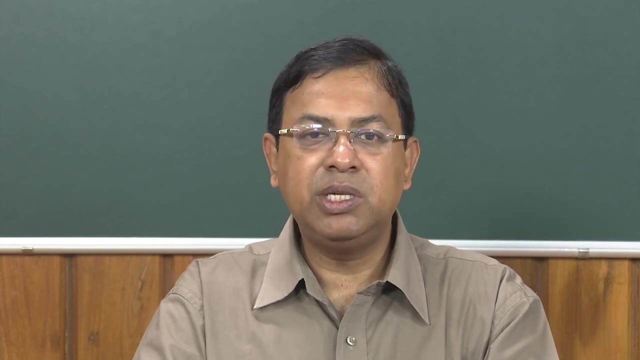 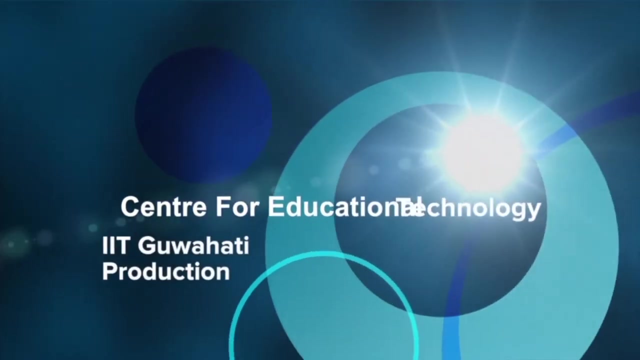 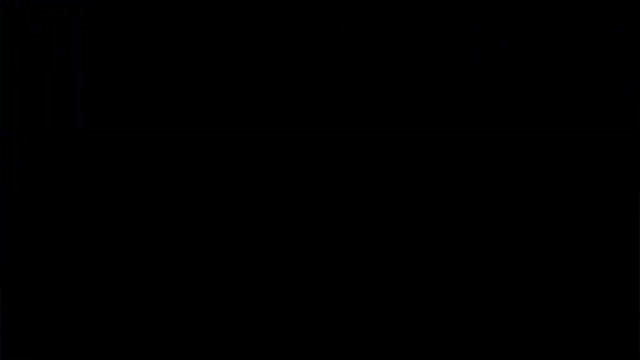 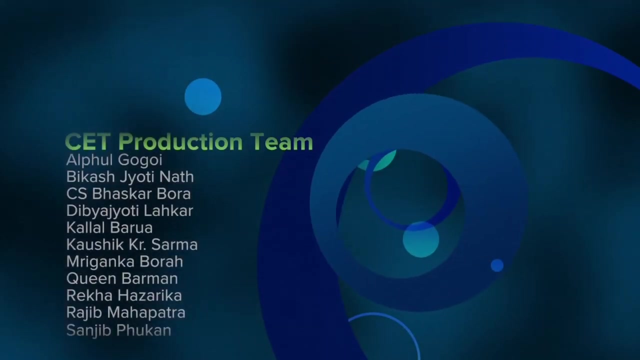 by a series of transformations which yield, finally yields: that this unknown state, quantum state, which is A up and B down, goes from lab A to lab B. Thank you.